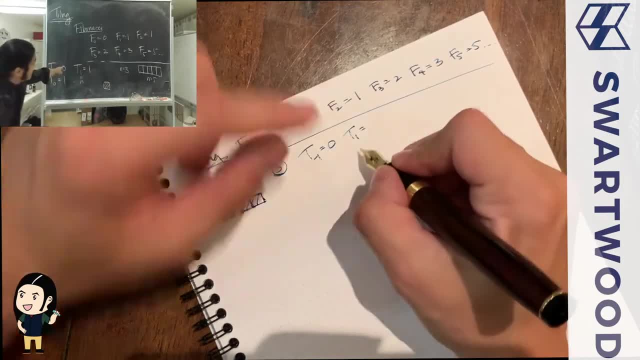 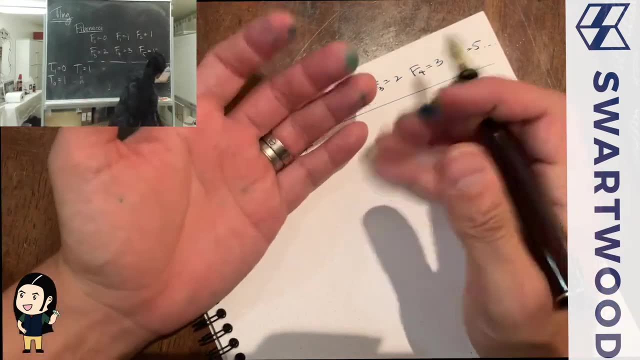 one is zero. you'll see why we're going to do this in a sec. and t of one. now t one we can actually think about. I'm sorry, t of zero, t of zero. we can think about. how many ways are there to cover a board that has nothing? there's only one way: you just don't do anything. Okay, now it gets. 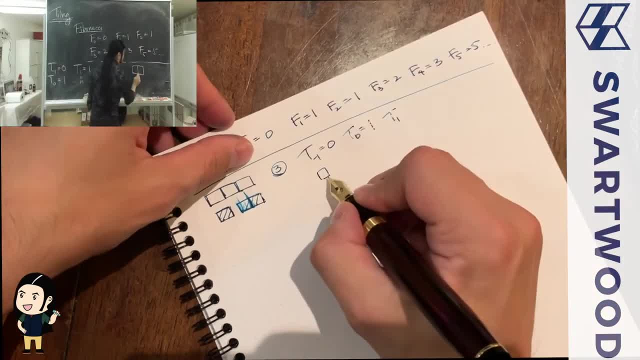 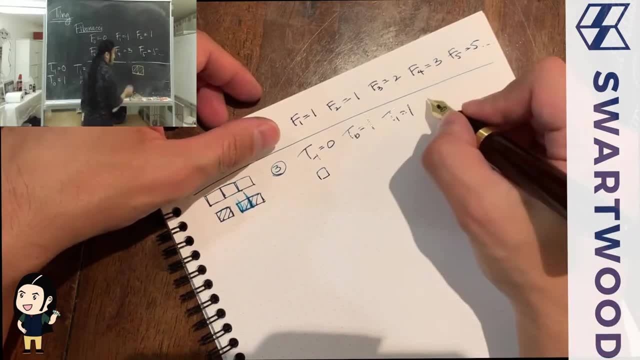 interesting. let's do t one. so our board has one square. how many ways can you cover that? there's only one way: you just drop a square on it, so it's going to be one square. Okay, how about t two? a guy that looks like this. how many ways can you cover this? well, there are. 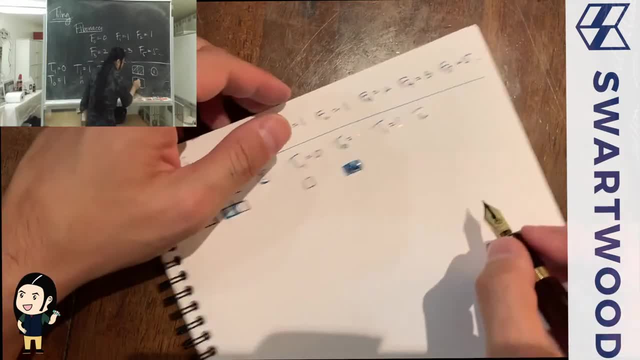 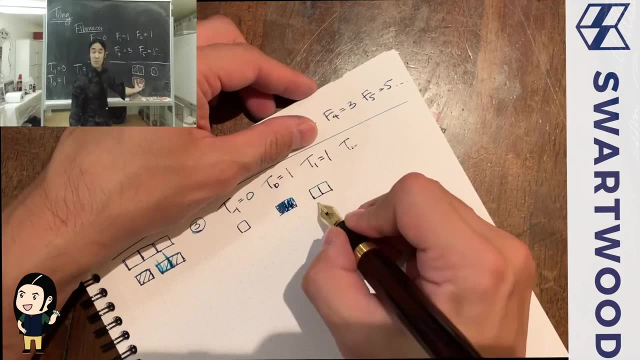 two ways. right, because you can cover it with a square. Okay, sorry, that was a failed attempt. again, I didn't think of a way of drawing this better. Okay, so let's talk about t two. how many ways can you cover this guy? well, you can cover it with a square and then a square. right, that's one way. 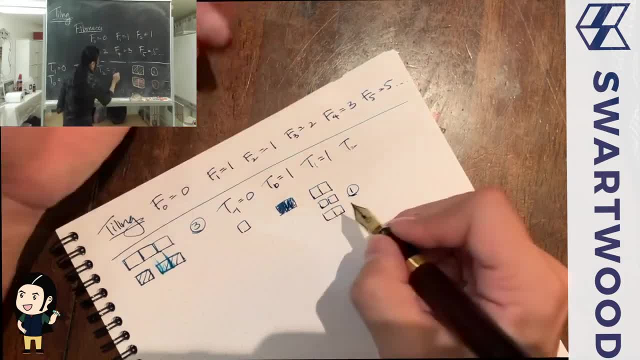 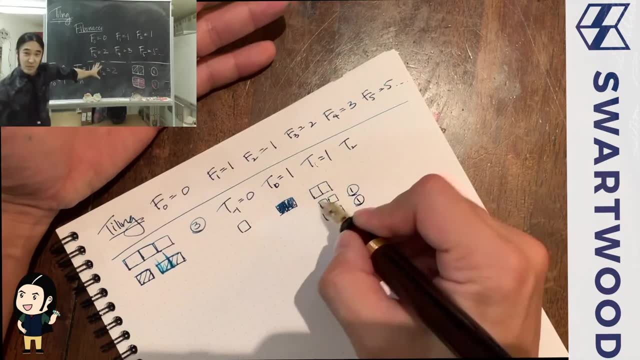 or you can cover it with a domino, which, I mean, just looks the same right, would look like this: Okay, so that's another way to cover it with a square, Another way, and I think those are the only ways to do it to cover this guy right? this we'll call. 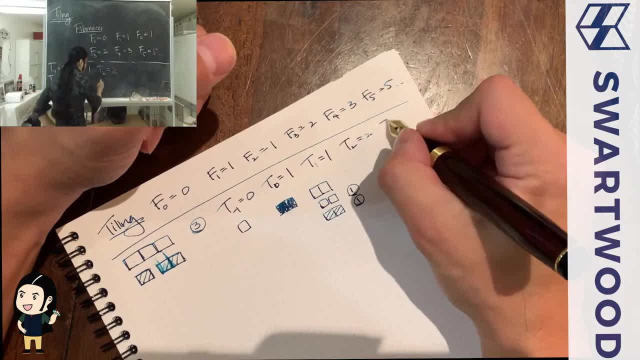 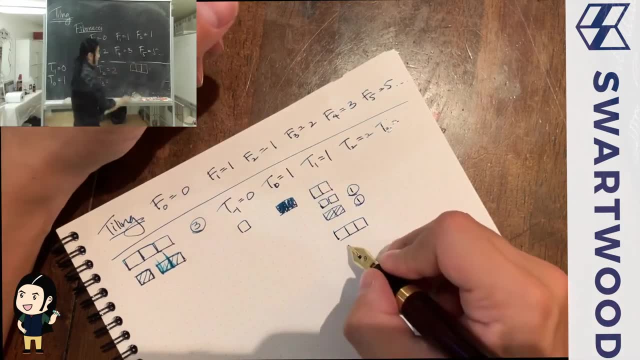 it a two board. so I guess there are two ways to do that. Okay, let's make it a little more interesting. how about t three? so if the board is composed of three squares, how many ways can you cover it? well, you can go square, square, square. that's one way. Okay, you could do domino, so let's draw a domino. 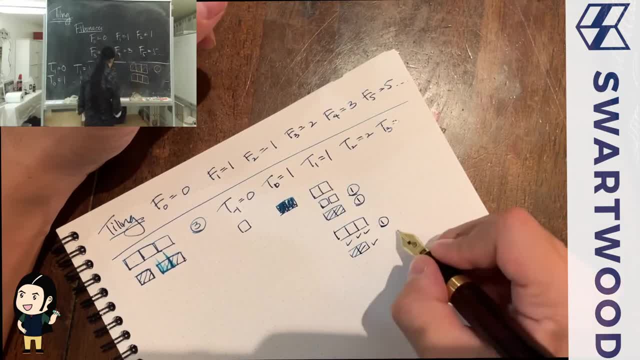 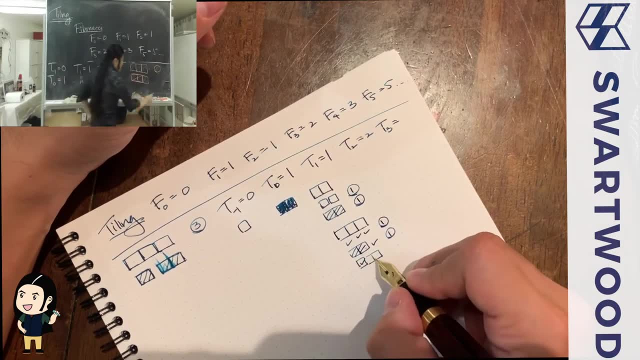 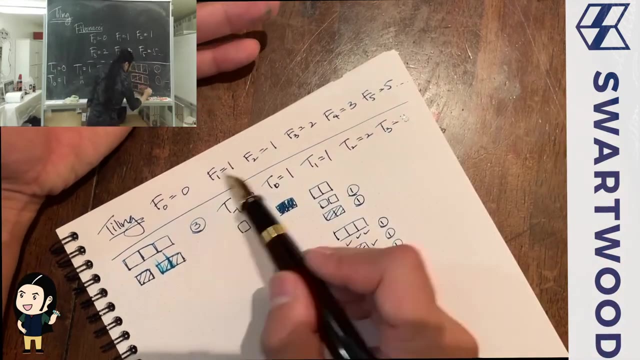 like this: you could do domino and then square, that's the second way, and then you can do square, square and then domino, that's the third way. so I think that's going to be three, but you can start to see a pattern here: zero one, one, two, three, five. zero one, one, two, three. let's see if this holds up. 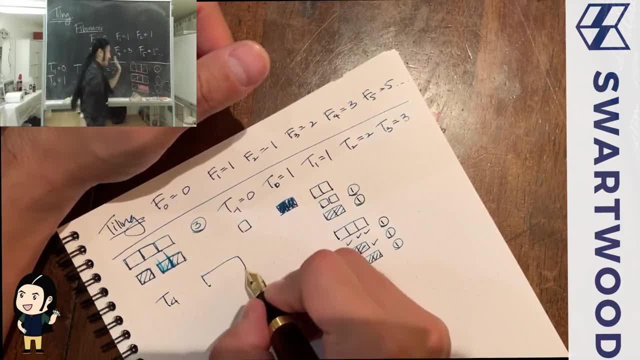 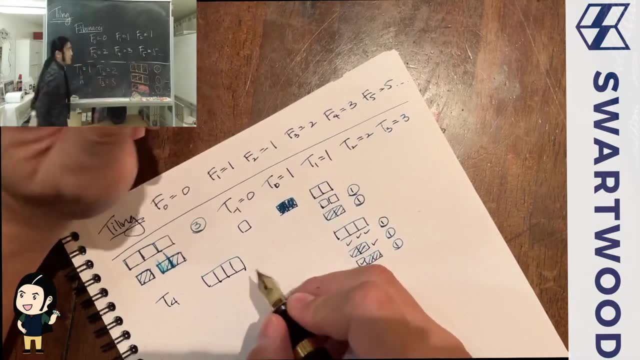 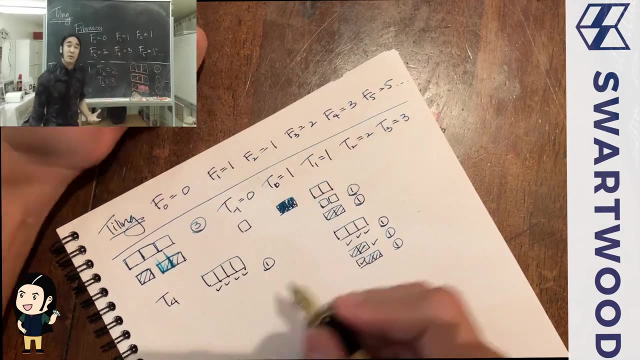 let's compute t four, okay, so I take this four board and see how many ways I can cover it, okay, well, um, just to make the notation easy, let's- uh, let's do it this way. one method is squares are going to represent with checks, So I'm going to do it: one, two, three, four squares. that'll work. okay, now it gets a little bit more. 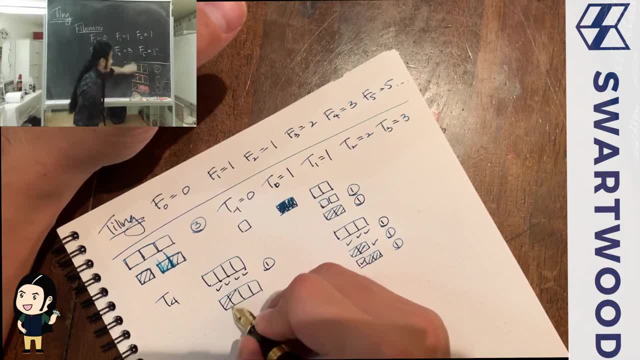 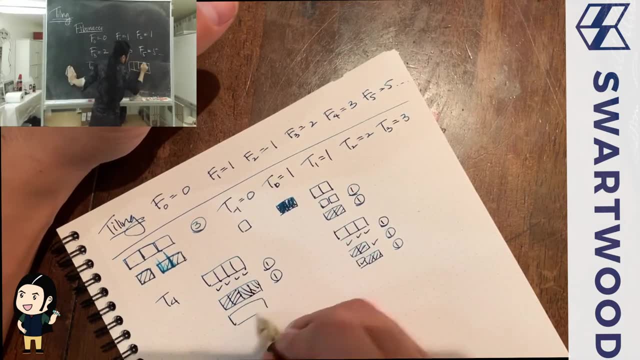 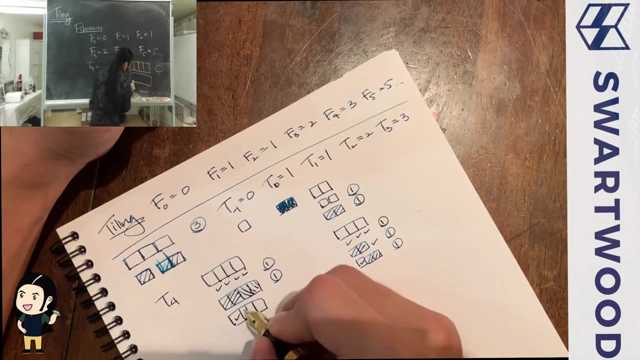 interesting. uh, we can cover this with, say, one domino like this and let's see another domino like that. that's another way, right, okay, otherwise, so it can be sorry, we can also do it this way. we can cover this with a square, a domino and a square. that's another way. we can also go. let's. 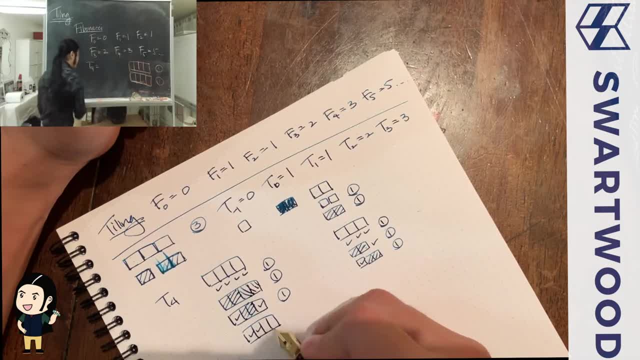 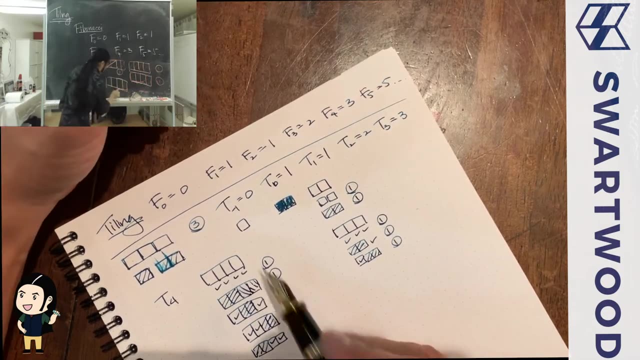 see, maybe, um, square, square, domino, right, and obviously we can go domino, square, square, okay, and if you think about it, I think these are the only ways we can do this. so there are five ways of doing this, so t4 is five, so there's definitely a pattern here and you can see. 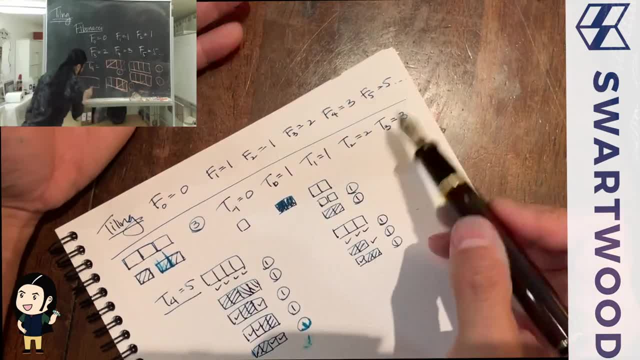 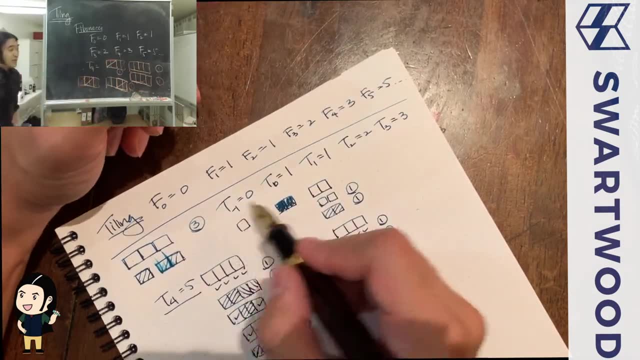 so this sequence looks just like the Fibonacci sequence, it's just that we're off by one, so t0 is one, whereas f of zero is zero in the Fibonacci sequence. so that's why I just artificially said t of negative, one and zero. okay, all right. so I guess entitled Lipton companies are helpful. 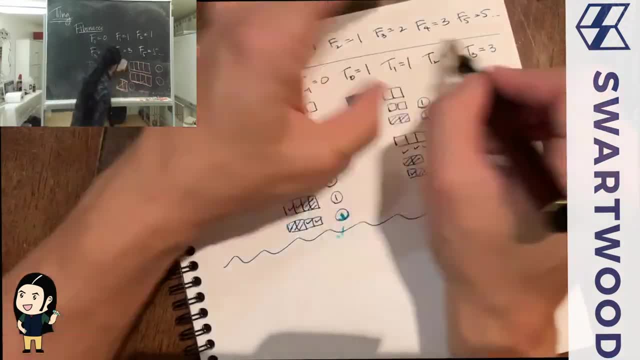 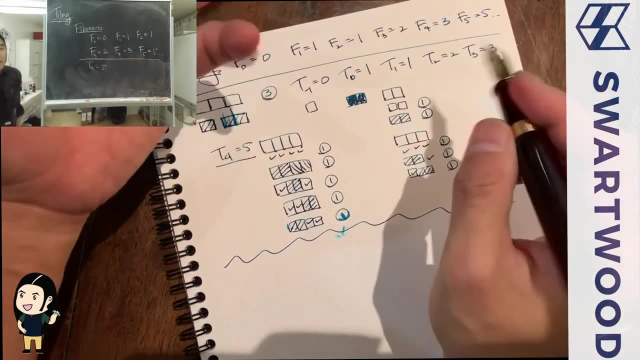 because some problems that might be more difficult to do. just strictly from the definition of the Fibonacci Sequence. you can do very nicely with tilings, okay. but before we get there, one thing is: why is this even true? because we know how the Fibonia sequence works. how do we guarantee that? 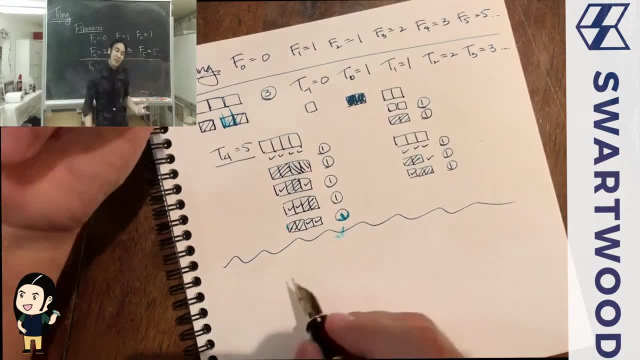 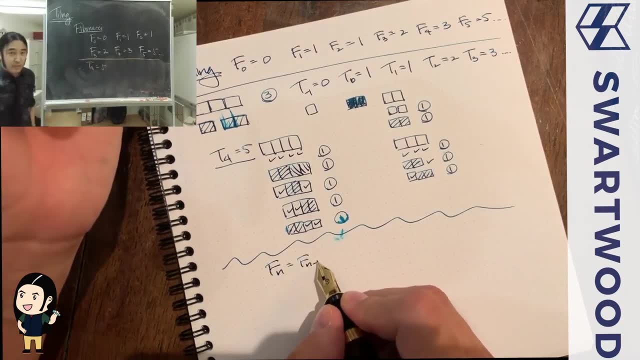 the Anatoly sequence works the same way, right for the one way. six, even though LMF, two tile sequence- same way, right? well, one way is this: if you look here, remember how we define the Fibonacci sequence: if you look at any guy, right, how do you get him? you look at one guy before and you add him to the 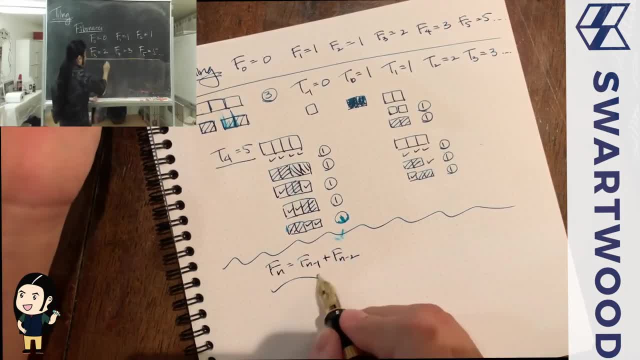 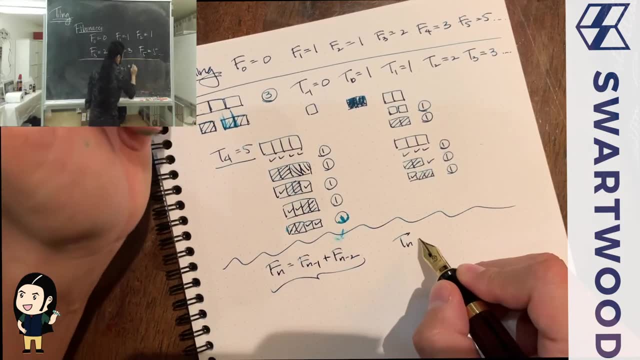 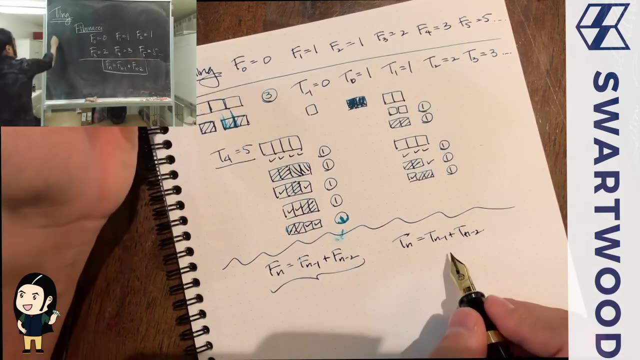 guy before that. okay, that was the key relationship. so now let's show that that's actually true for the tiling guys, because if it's true that tn right is equal to tn minus 1 plus tn minus 2, then the patterns look the same. right now it's not exactly true because the the indexing is off. 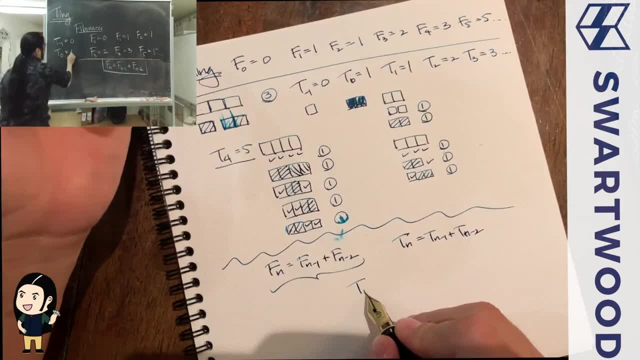 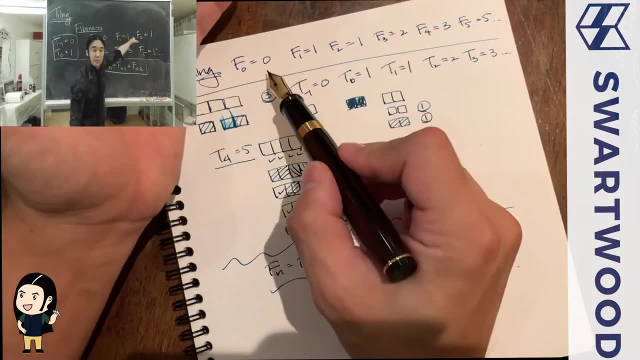 but that's easy to fix. we just say that t of n right is equal to f of n, plus 1 right. t of negative 1 is f of 0, and we set it up so initially you have 0, 1, 0, 1. they're lined up, so as long as you. 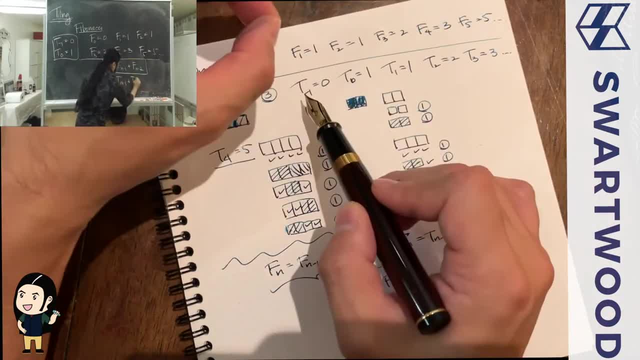 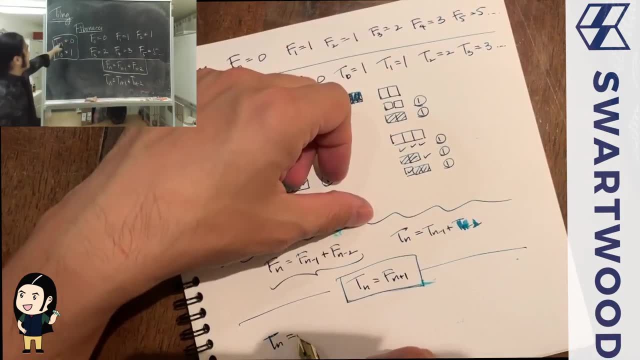 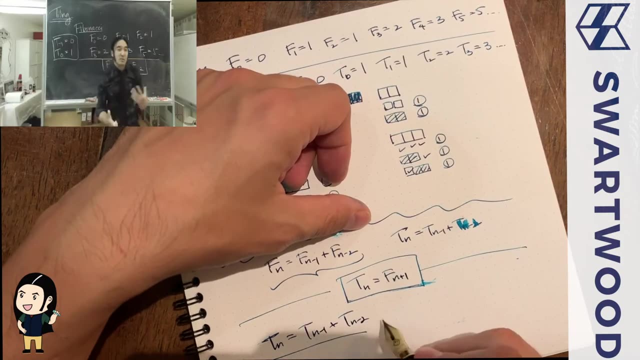 construct these guys by adding the previous two and you construct these guys by adding the previous two. we know the sequences are going to be the same, okay, so all we have to show is this relationship: okay, okay, tn. t sub n- sorry- is equal to t sub n minus 1 plus t sub n minus 2. that this holds, okay, sorry. 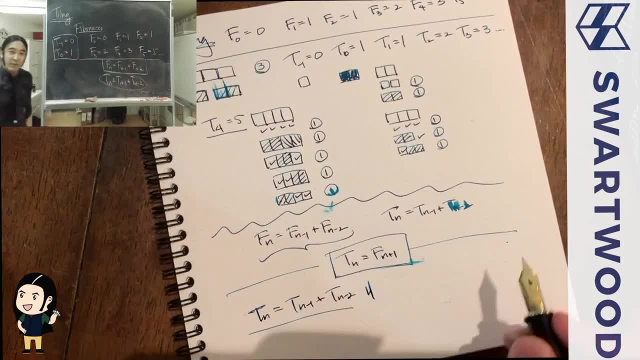 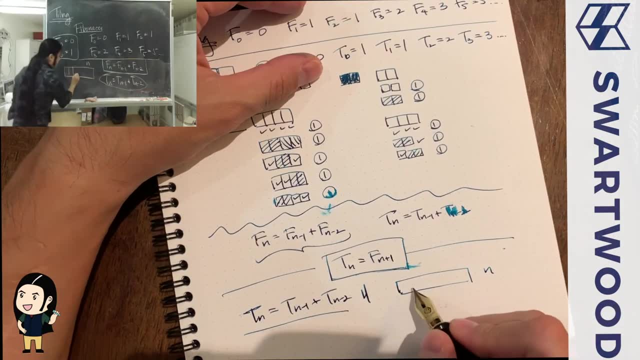 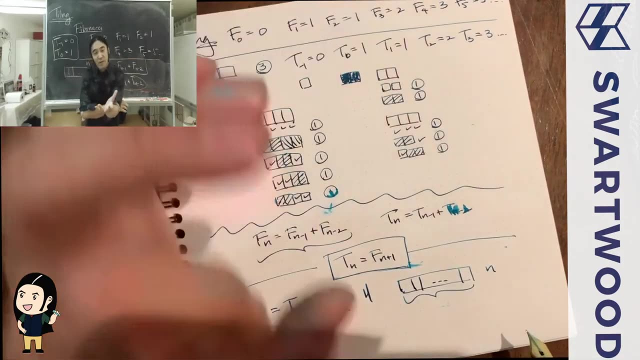 i think we're running out of ink. okay, all right. so how do we know that we're going to do a tiling argument? so imagine you have some n board, okay. so let's think of. imagine all the different ways there are to tile this n board. okay, you can really break it on this way. no matter what we do, we've 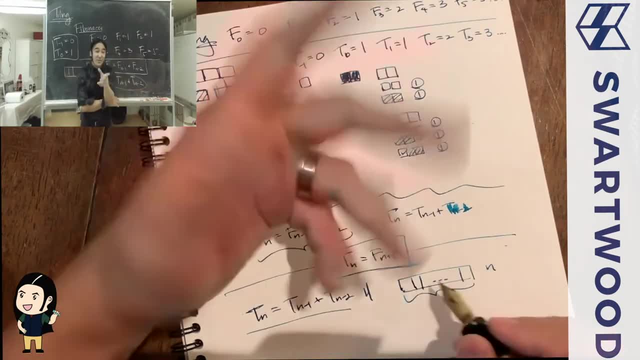 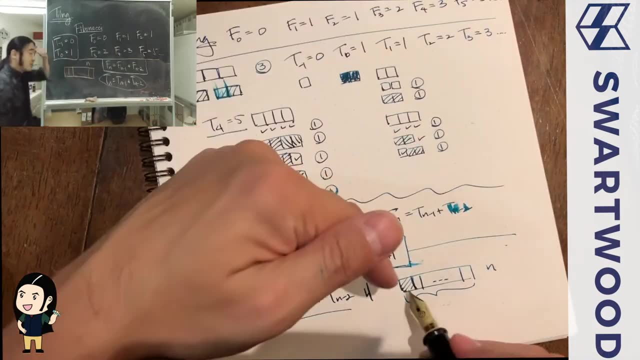 got to cover this n board, okay. so let's think of imagine all the different ways there are to tile in front of the square right, and i think we've already covered this first square right. so one obvious way of tiling this thing is to literally just tile that first square, okay. so what are the? 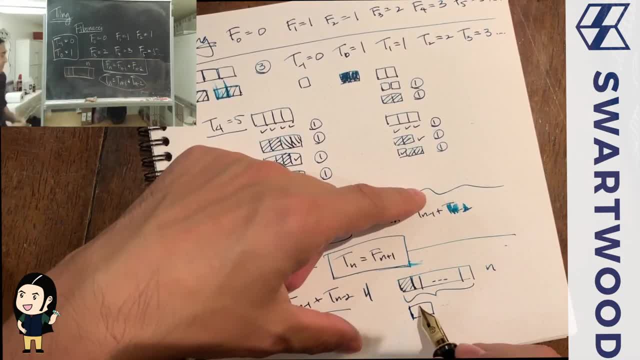 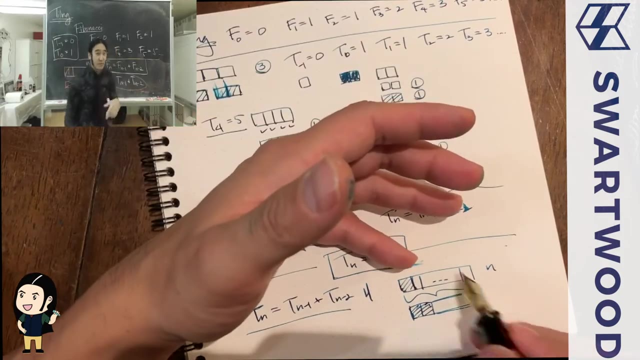 options. you need to cover that for a square. there are only two ways to do it. you can either cover it with a square or you can cover it with the domino. uh, okay, like this, does everybody agree? and then the rest of this go on. okay, so those two cases cover. 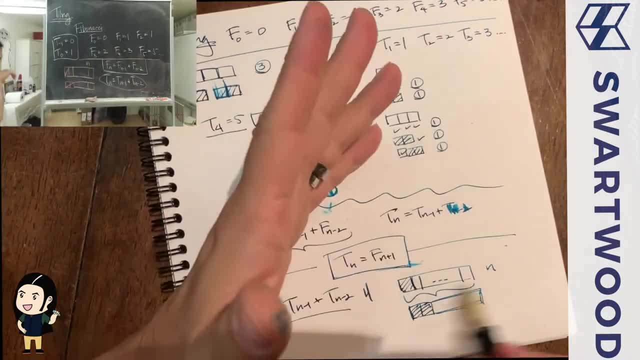 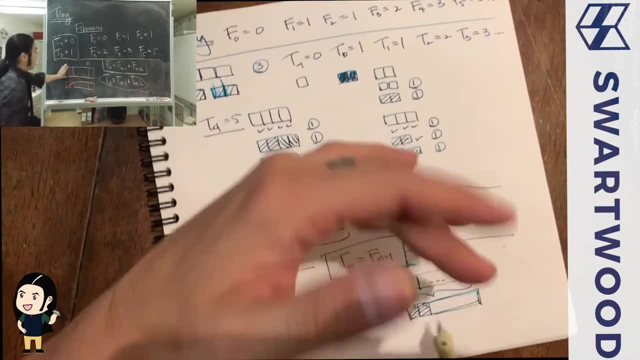 everything. now. i know there's a bunch of junk going on here, but it's always got to be a case to cover square one. So if you look at that end board, the first square on the end board must be covered And you can cover it with a square tile- I should have said tile before, right, Or you can. 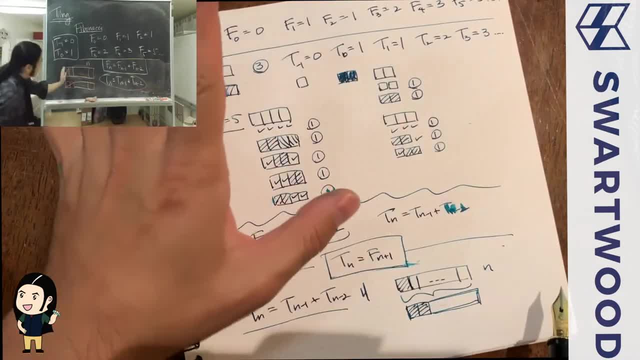 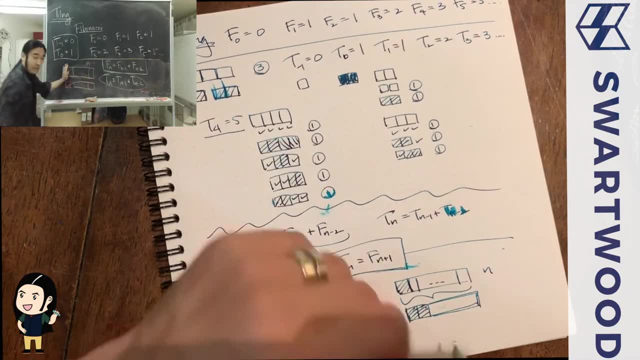 cover it with a domino. Okay, So those are the only ways to do it. So you can literally break everything down into these two cases. Okay, Count the number of ways you can do this starting with a square, Then we'll see the number of ways you can do it starting with a domino, And we'll put 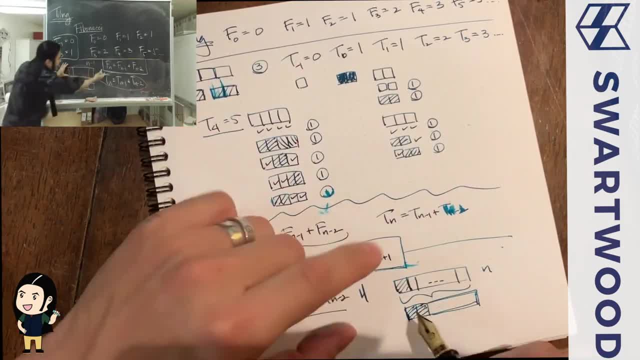 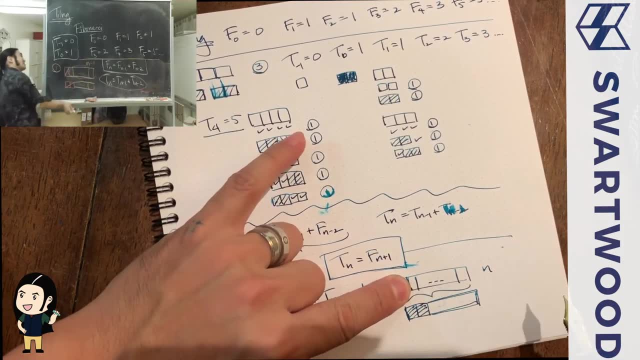 all those cases together and we'll get the answer. But this is actually pretty fast, because if you covered this guy with a square right, What's left? Well, anything can happen over here. So this is like tiling a regular board right. But what's the size of this board? It's n minus one. So the number 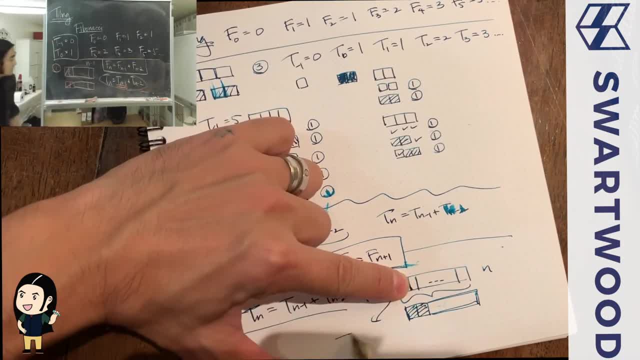 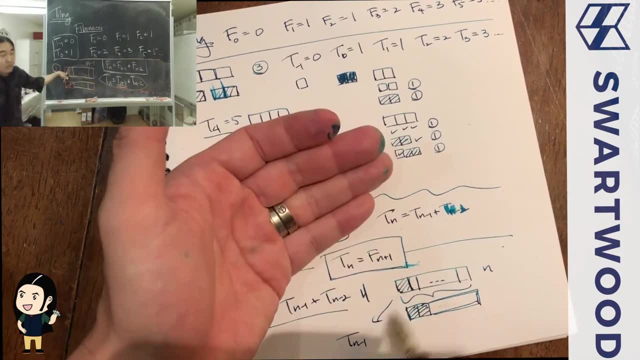 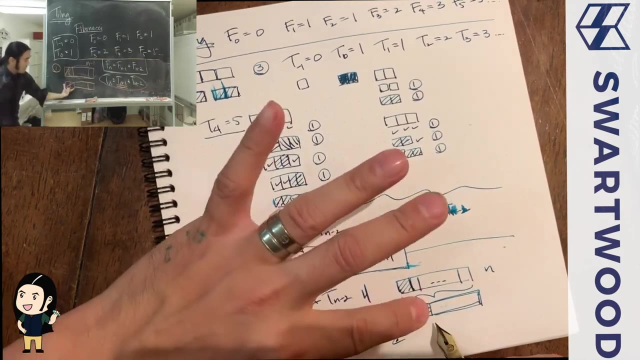 of ways of covering this guy is actually tn minus one. So imagine all the ways of covering an n minus one board. tack on this guy at the end and you've got what A covering of an end board. Okay, Now let's do it for this thing. Sorry, I erased that board over Once we put down this domino, how many?